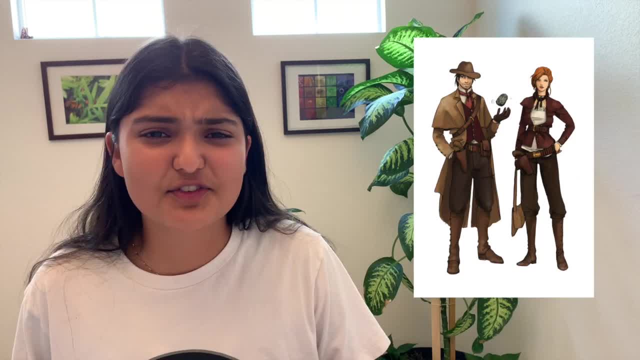 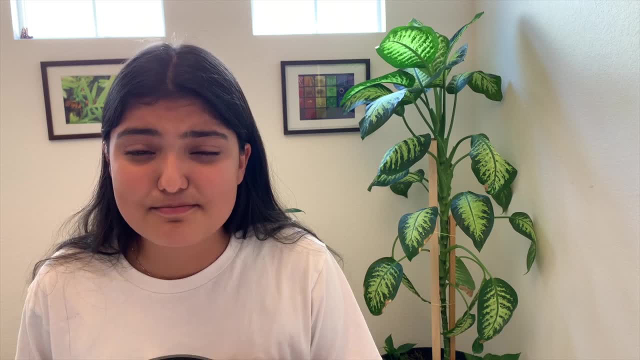 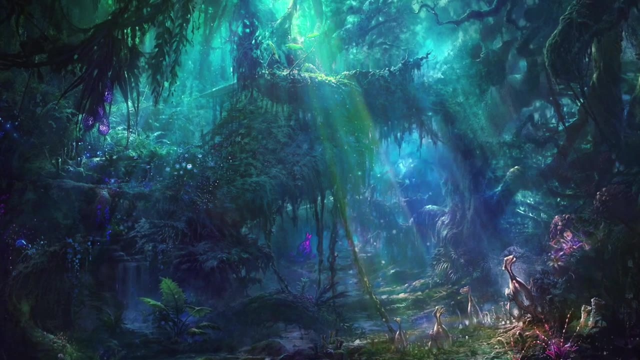 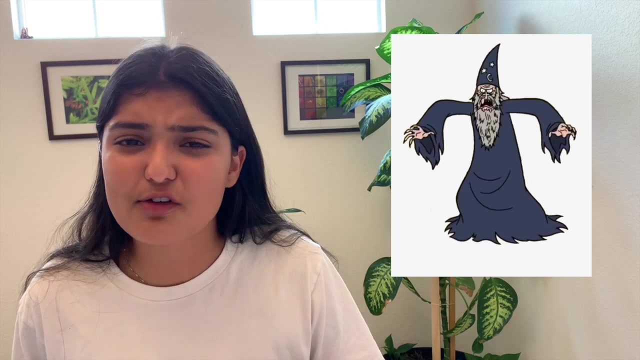 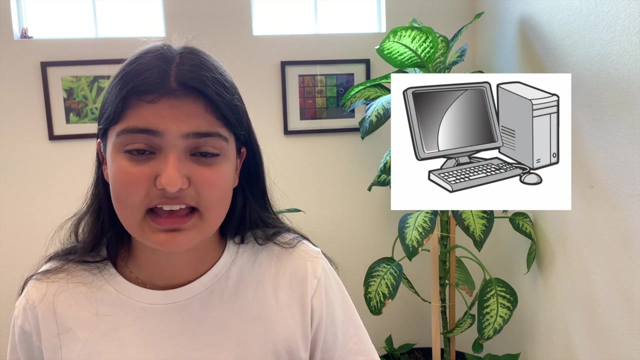 Today you're an adventurous human and for some odd reason, you find yourself walking through an enchanted, mysterious, mystical forest. Suddenly, you come face to face with an evil magician. All of a sudden, he pulls out his evil magician staff and points it at you, turning you into a computer And to torture you even. 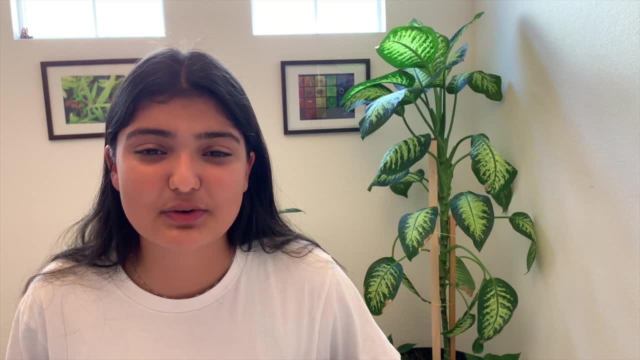 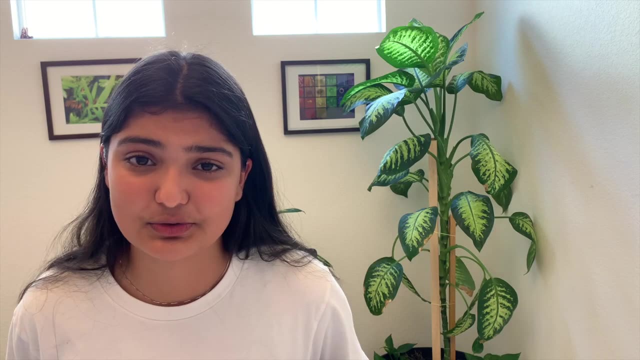 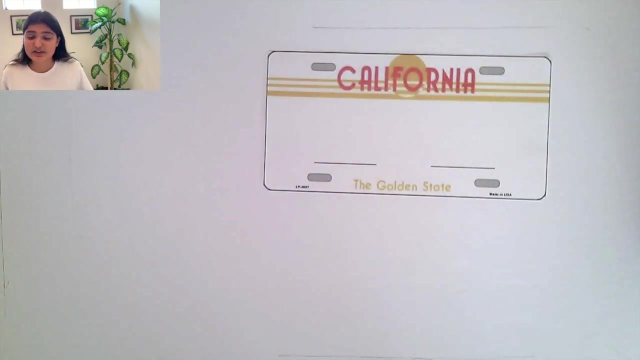 further, he turns you into a computer who generates license plates for the back of cars. Brilliant, In fact, I got turned into one too, So let me show you. Yesterday, I generated this license plate, or one that looks like this, and the only rule I had was to make sure that it was composed of: 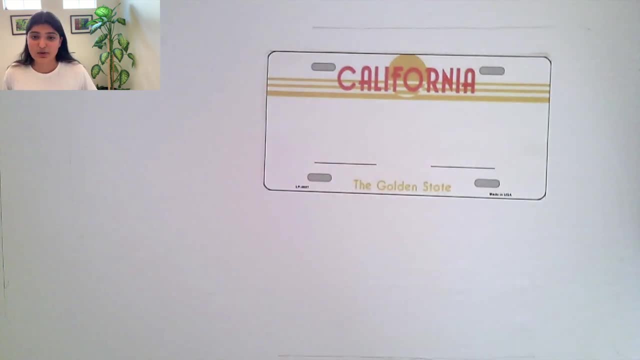 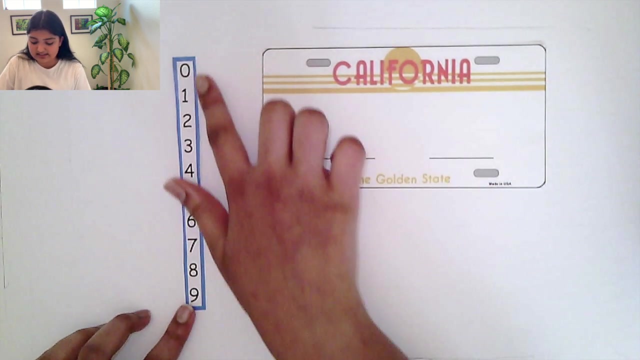 two characters that had the same license plate. I had digits between 0 and 9.. With the rules, I was able to generate so many license plates. Let me show you how. In the first place of this license plate, I had 10 different digits I could choose. 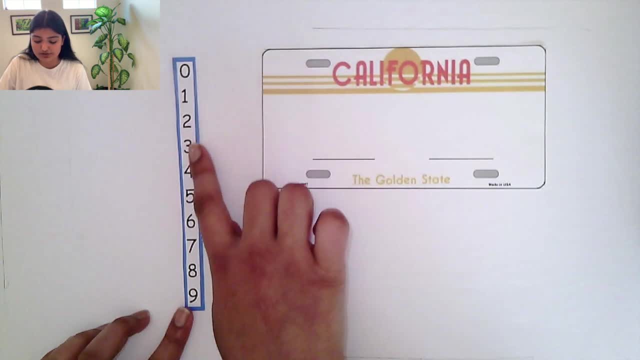 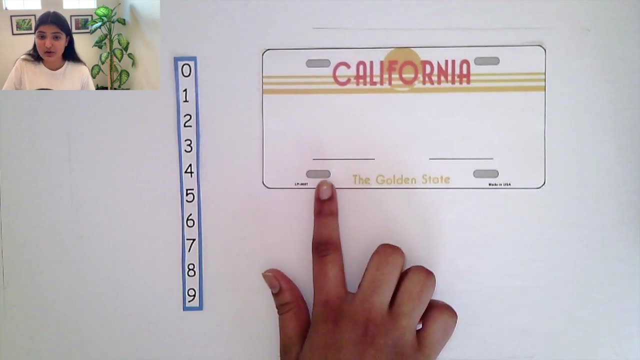 from 0,, 1,, 2,, 3,, 4,, 5,, 6,, 7,, 8 or 9.. After I chose one of these digits, from any of zero to nine, i had nine different digits that i could choose from for the second place. 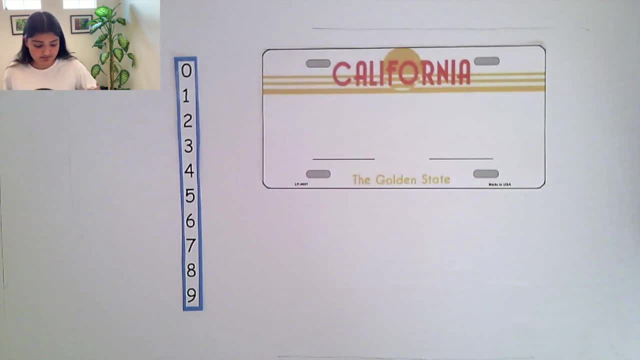 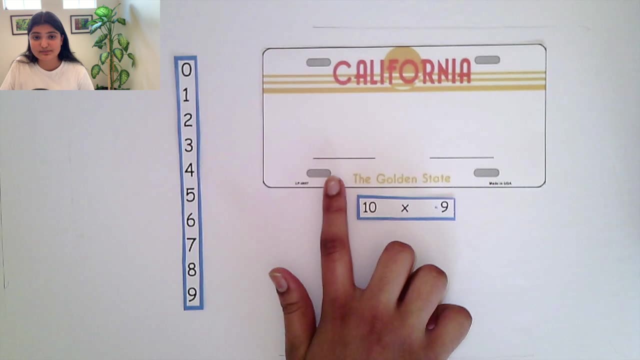 so how many possible license plates could i have made? well, i had 10 possible options for the first place and nine possible options for the second place. this led to a total of 90 possible license plates. that i couldn't make well, good news though i have. 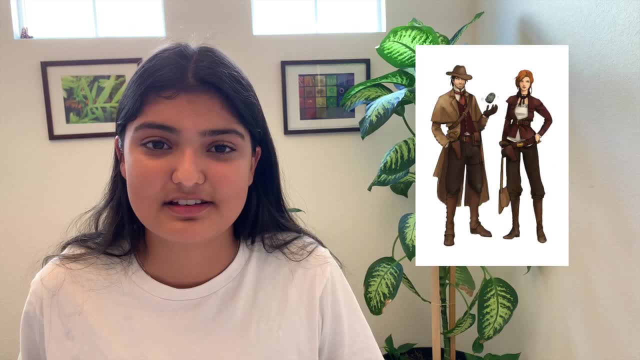 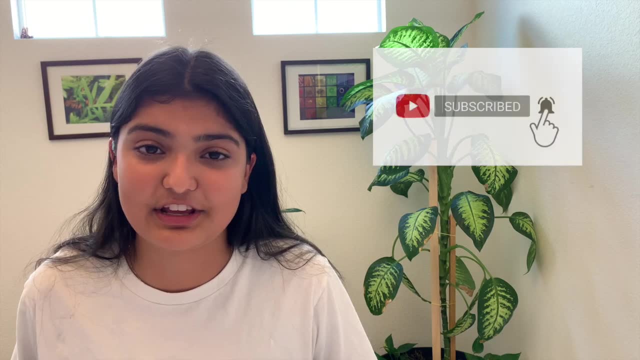 the cure to being turned back into an adventurous human. all you have to do is like subscribe and hit the bell to receive notifications for every time we upload a video. but while we're still computers, let's get back to generating license plates. here's today's issue. 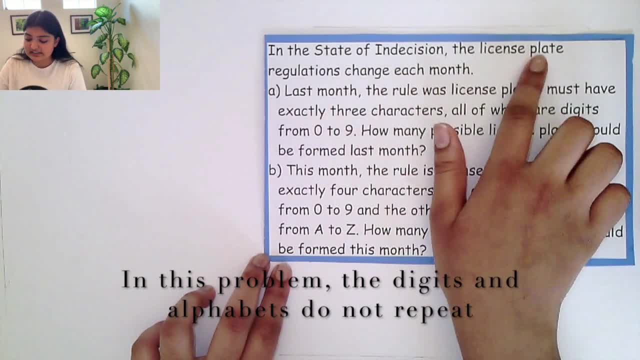 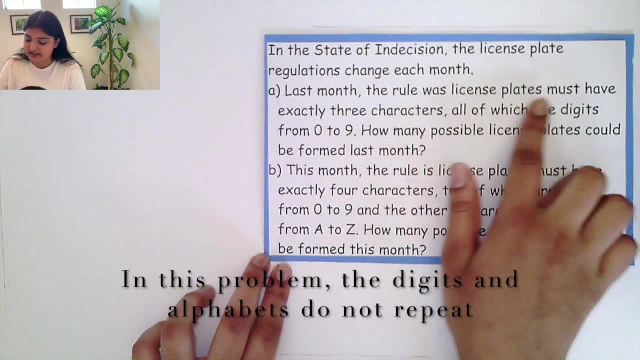 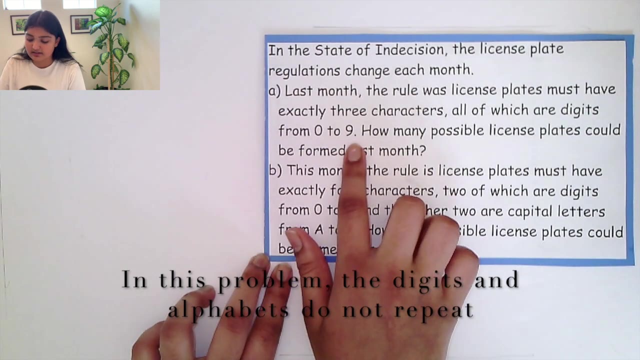 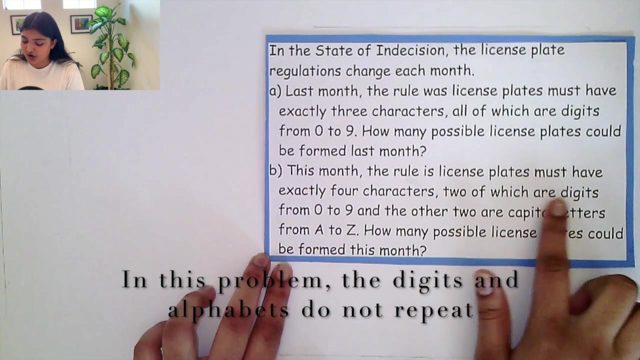 in the state of indecision. the license plate regulations change each month. last month, the rule was license plates must have exactly three characters, all of which are digits from zero to nine. how many possible license plates could be formed last month? this month, the rule is license plates must have exactly four characters, two of which are digits from zero. 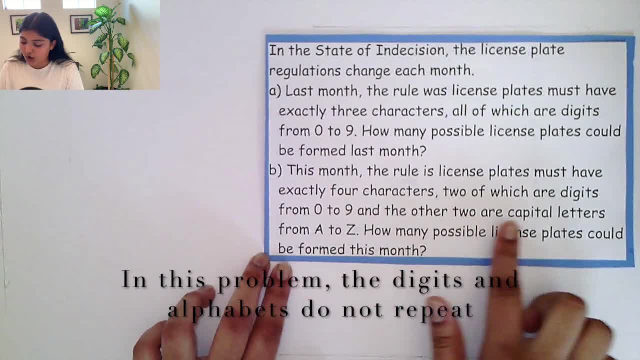 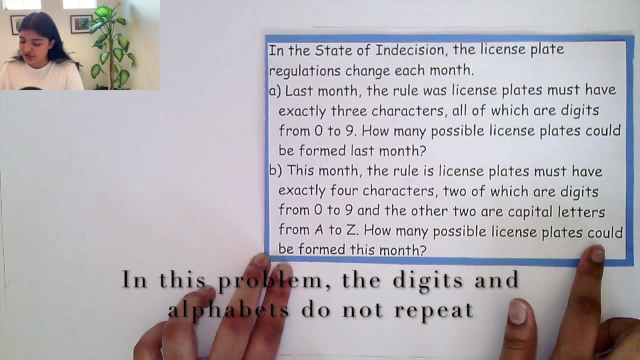 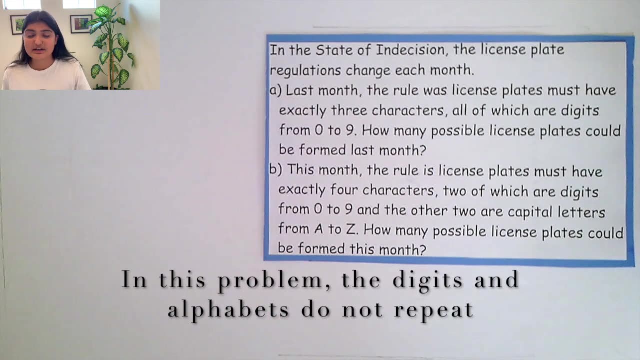 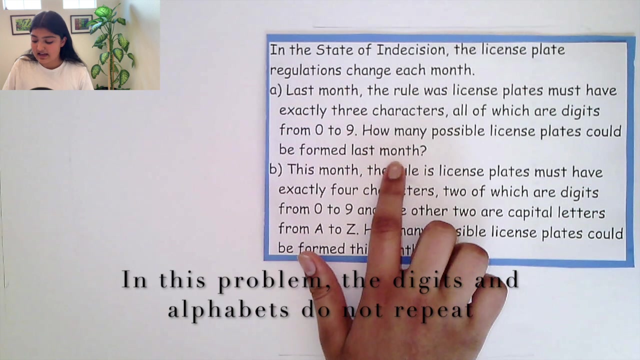 to nine and the other two are capital letters from a to z. how many possible license plates could be formed this month? by rereading the problem and the issue of today, we can see that we have to solve for the total possible license plates from last month, as well as a total possible license plate that could be. 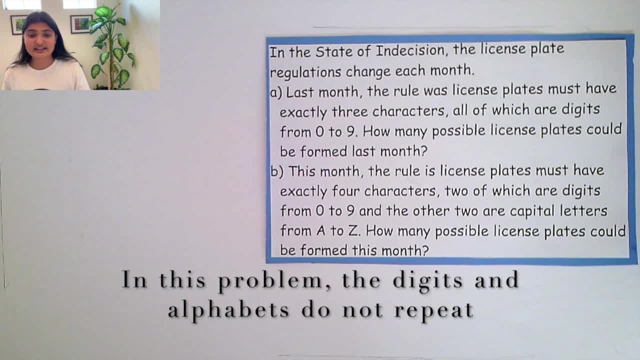 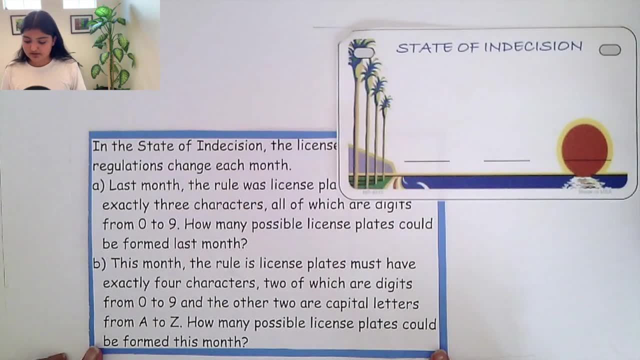 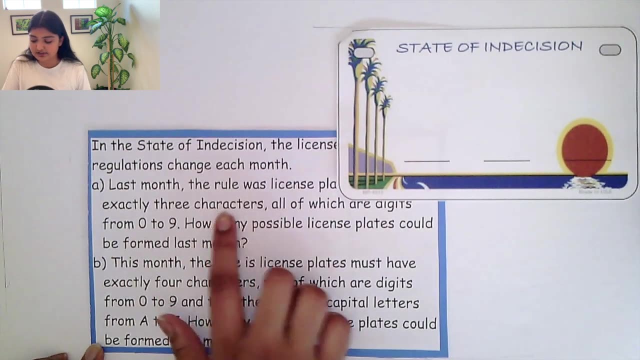 formed this month. so let's start by finding the total license plates that could have been formed last month. turning back to the problem, we can see that the license plate must be composed of exactly three characters, as shown here. all three of these characters must be any digits between zero to nine. 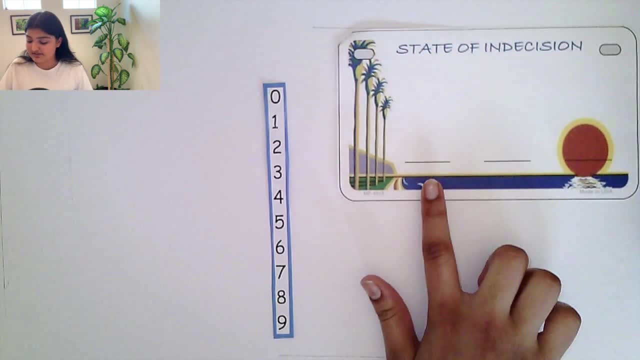 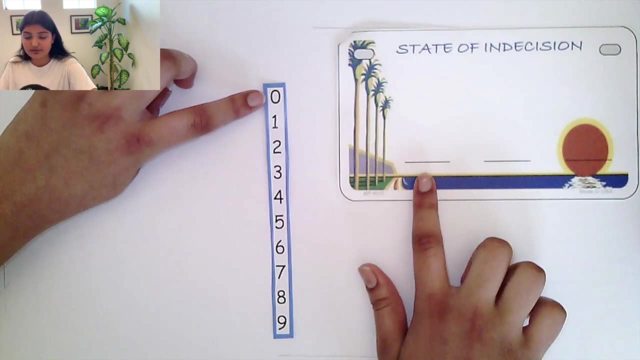 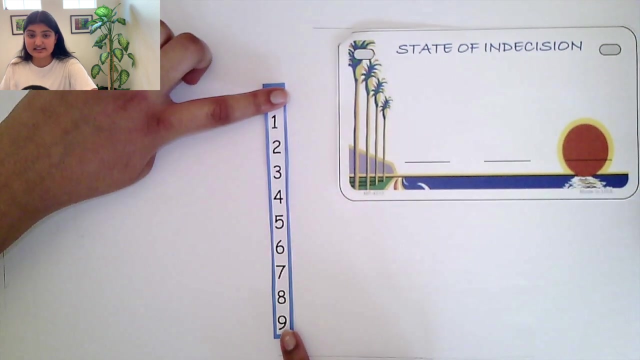 let's start with the first place. the first place of this three digit license plate can have any one. Suppose we choose 0 for the first place, The second place can have any one of these nine digits, as one of them is already taken for the first place of this. 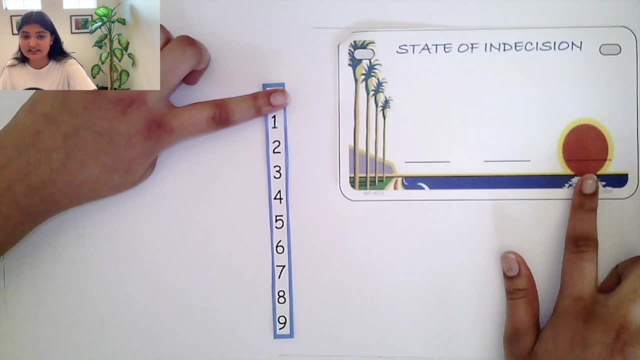 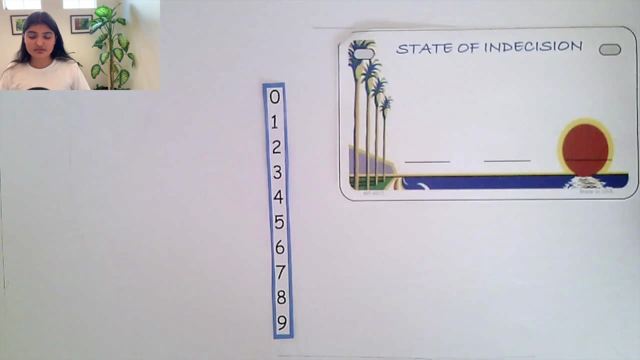 three-digit license plate. And finally, the last place can choose any 8, as the first two digits were already taken. So how many possible license plates can you make? Well, we can multiply 10 times 9 times 8.. Remember, for the first spot there were 10. 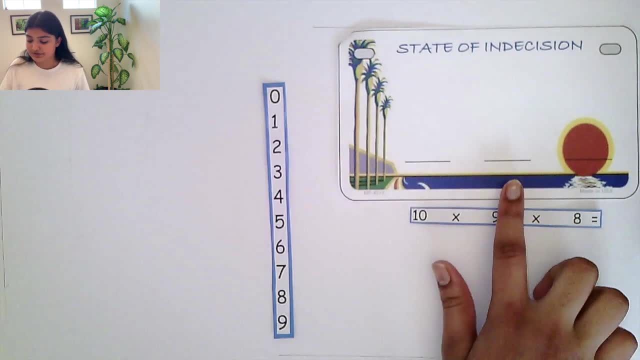 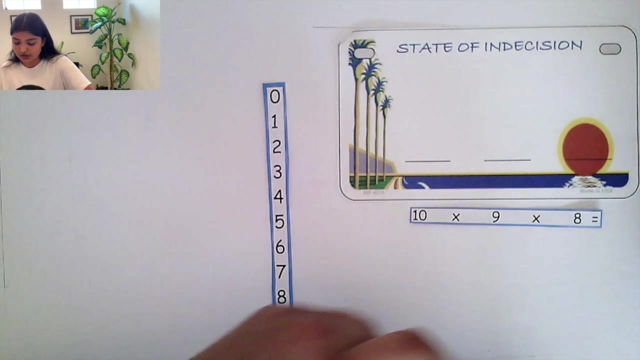 different things between 0 to 1.. For the second spot, there are nine different digits, as one has already been taken, and for the last spot, there are eight different digits, as two have already been taken. We can multiply by this to get a total of 720 possible license plates that could have been created in the state. 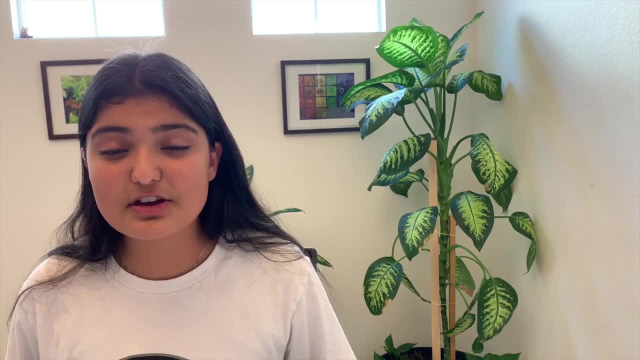 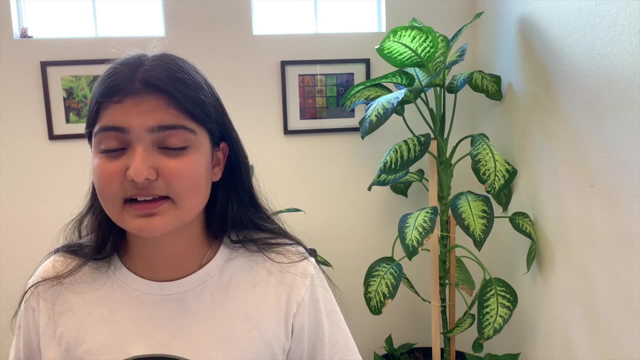 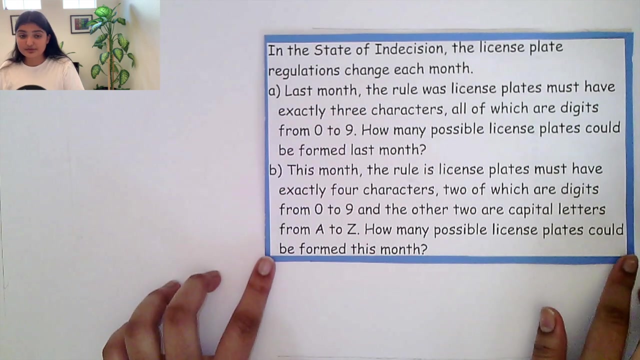 of indecision last month. Now that we know the total possible license plates that could have been created last month, let's go back and find the total possible license plates that could have been created this month. Looking back at the problem, we can see that this month license plates 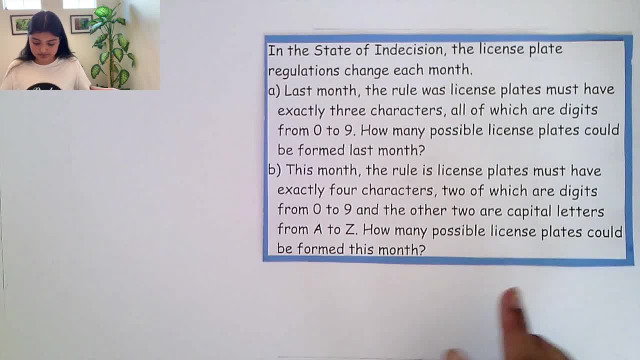 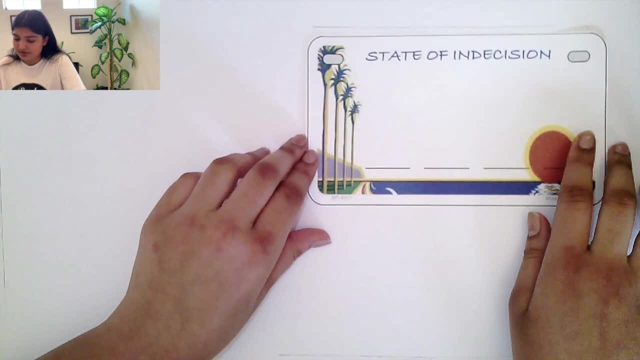 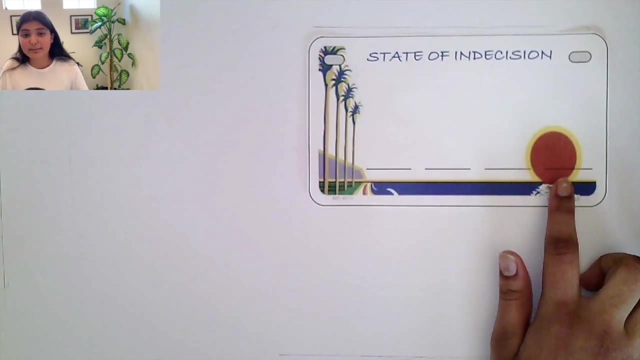 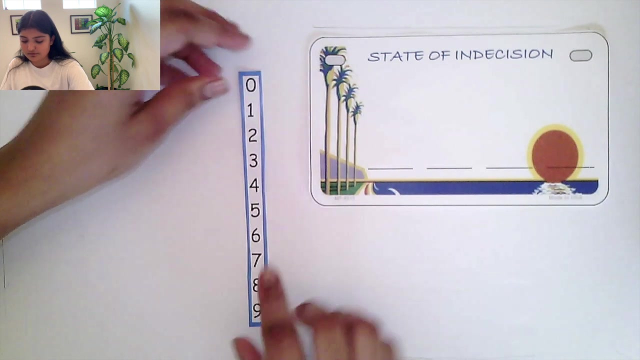 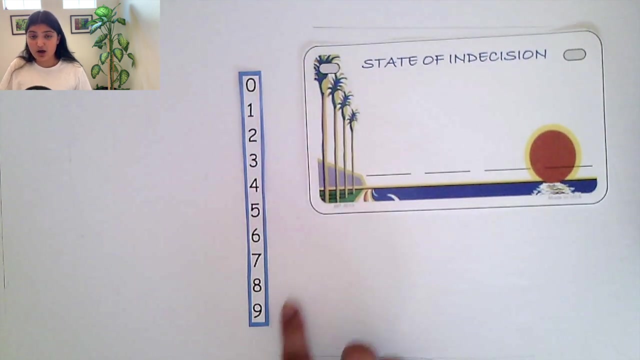 must have exactly four characters. Two of these must be digits, while the other two may be any capital letters. So let's find how many possible license plates we can have. Well, for the first two, we can use any one of these 10 digits. Therefore, for the first place, we have 10 different options. 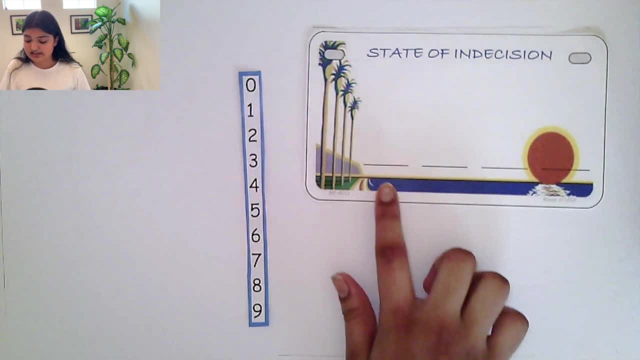 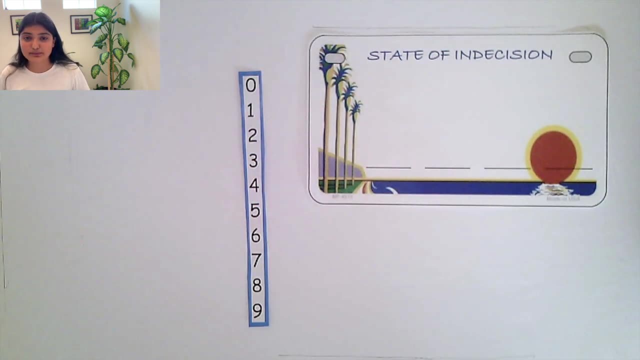 For the second place, we have nine different options, as one of them would have been taken to fill the first column. Therefore, we have nine different options. Therefore, we have nine different options. Therefore, we can start by finding the total possible. 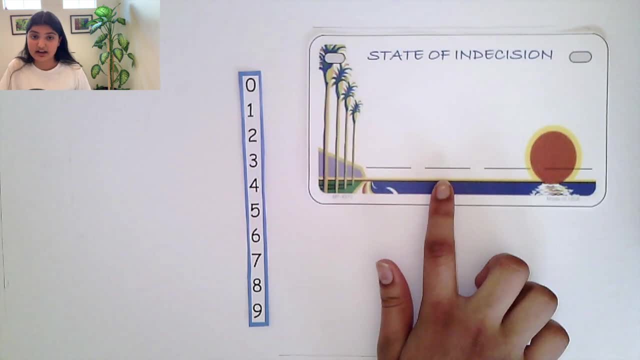 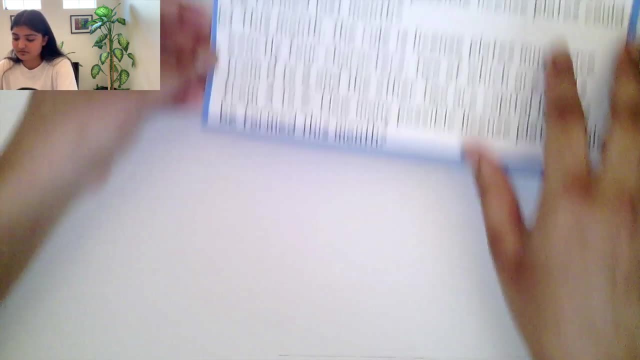 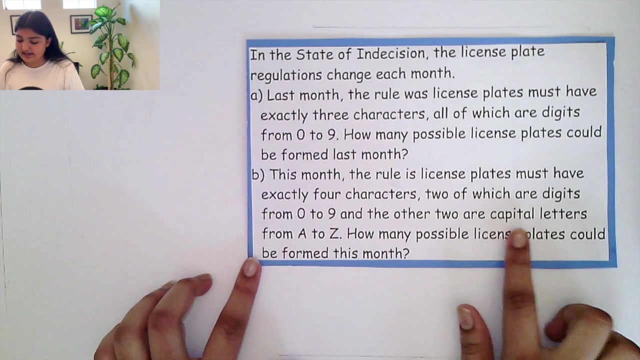 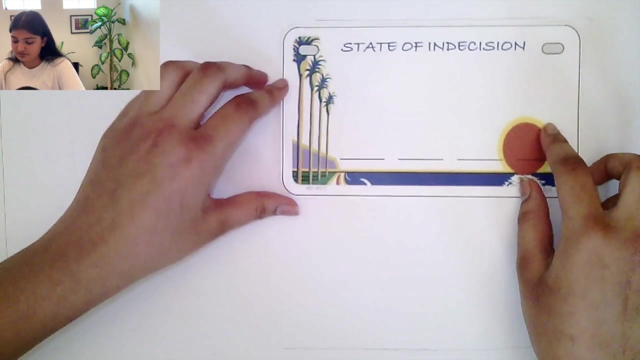 license plates by multiplying 10 times 9.. Now let's look at the second part of the question. The last two characters of the license plates must be capital letters from A to Z. The last two characters of the license plates must be capital letters, from A to Z. 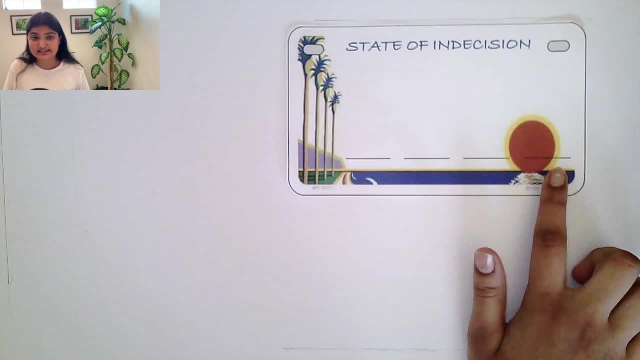 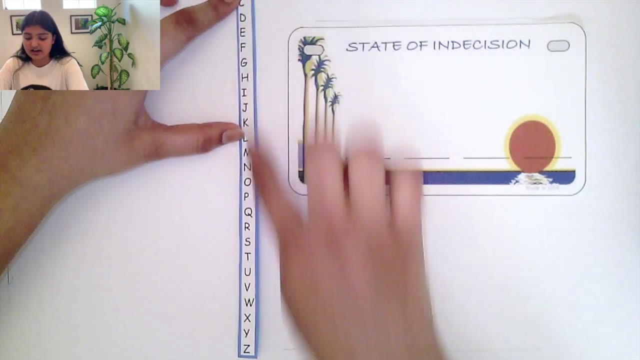 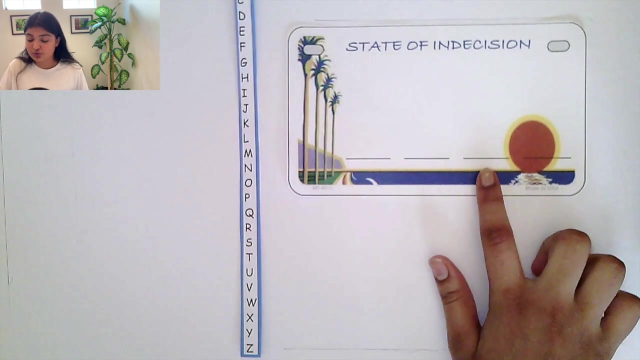 Here we have the last two places of this four character license plate. As we can see, they can be any one of these letters from A to Z. Since there are a total of 26 letters in the alphabet, there are 26 possible letters that.